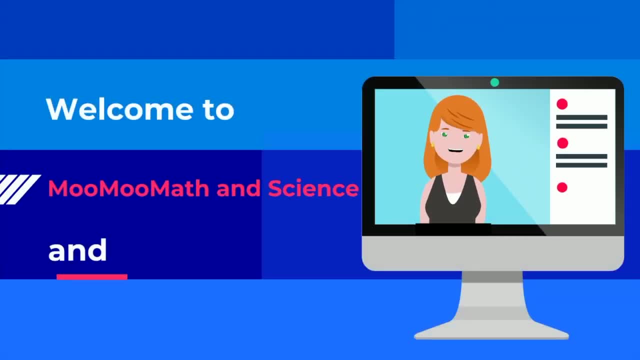 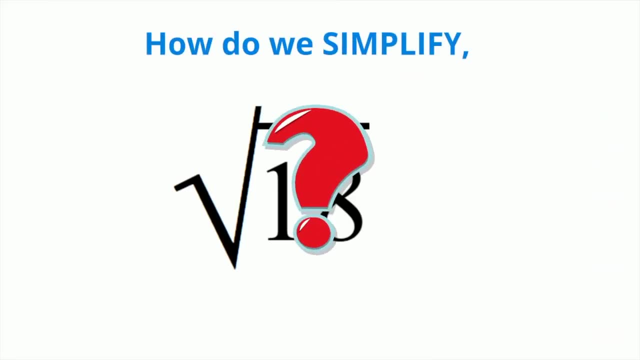 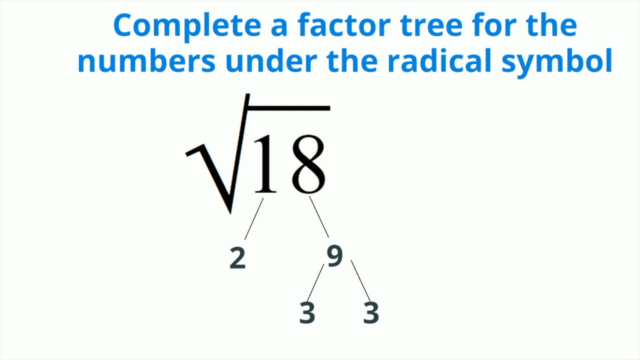 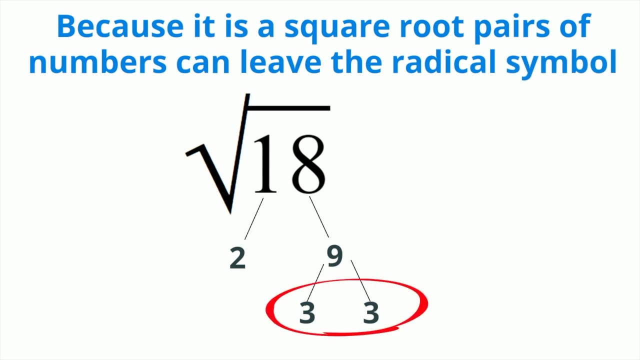 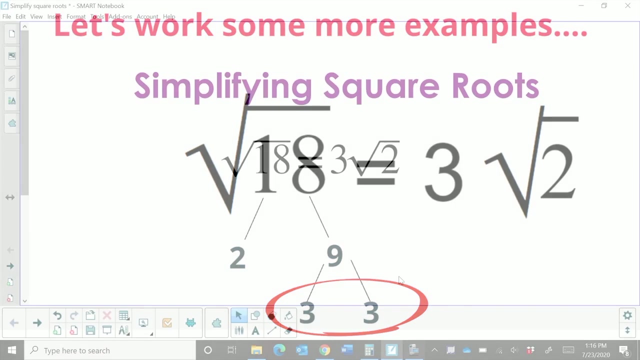 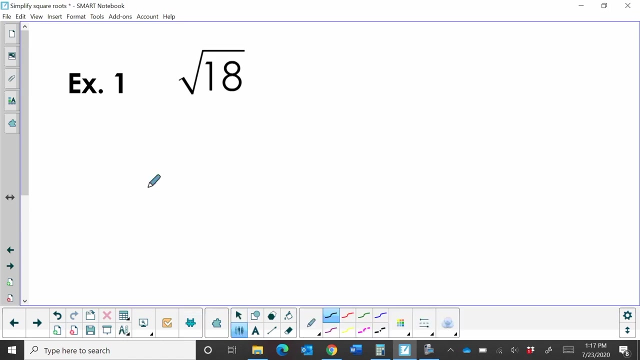 Subscribe. We're going to look at simplifying square roots. So let's look at how you would simplify the square root of 18.. So what do I do? What I do is I actually create a factor tree, Because this is an even number. I just divide it by 2.. 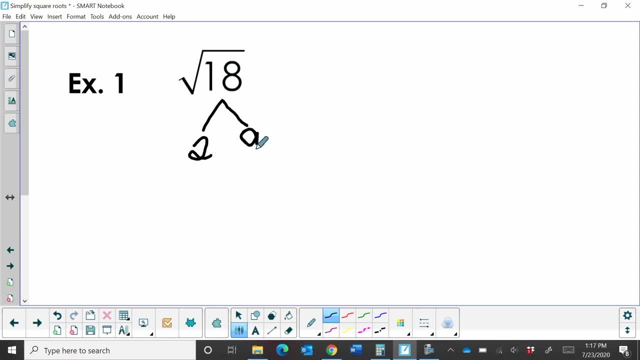 I make it very simple: 18 divided by 2 is 9.. Then I take the factor. Well, 2 won't factor because it's prime. The only factors it has is 1 and itself. but 9 factors into 3 times 3.. 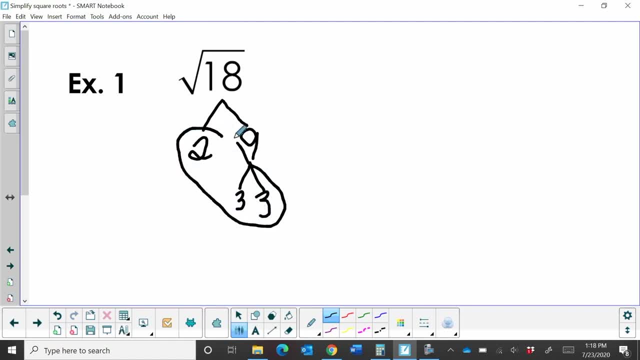 So now what I've got is: I've got these prime factors right here. So the prime factors of 18 are 2 times 3 times 3.. And since this is simplifying a square root, I know that 9 is a perfect square. 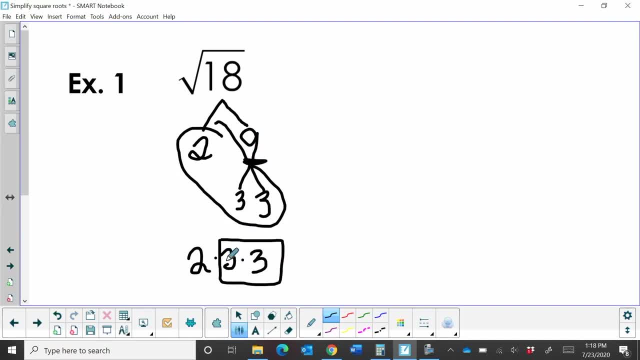 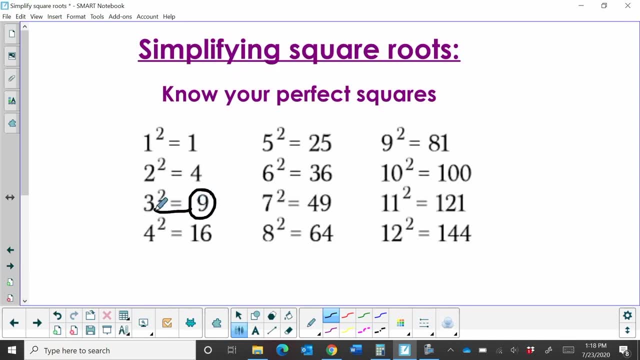 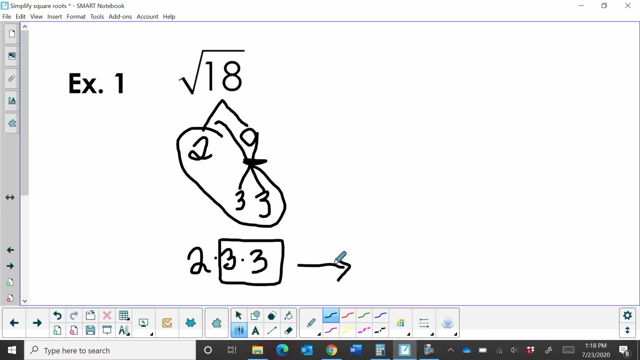 So 9 is perfect square And it factors into 3 times 3.. So basically, what I'm doing is I'm finding this perfect square and I'm simplifying it back to its square root. So this will simplify to 3 square root of 2.. 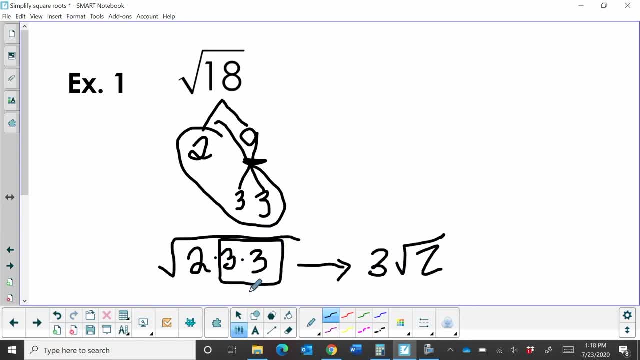 Because all of this actually is under a radical. So the square root of 9 is a perfect square. It factors into 3 times 3.. The 3 times 3 is a perfect square. The 3 comes out because it's a perfect square. 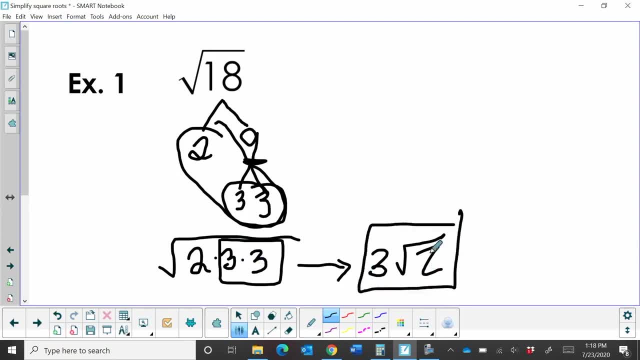 And the 2 stays in because it is not a perfect square. So that's how we get 3, square root of 2.. So let's try a second one. Let's try square root of 24.. So again, it's even. 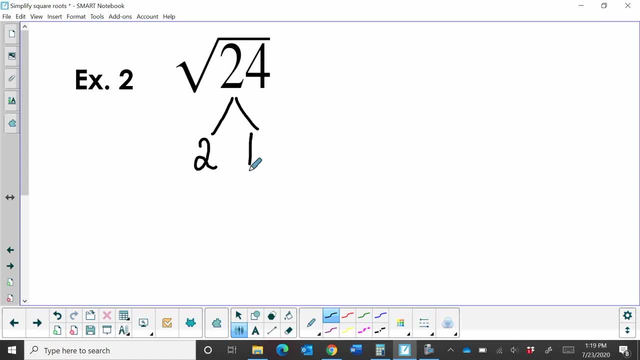 So let's break it down to 2 times 12.. Okay, 2 is prime, so I don't have to worry about that. So let's factor it again 2, because it's even again times 6.. Well, 6 is even. 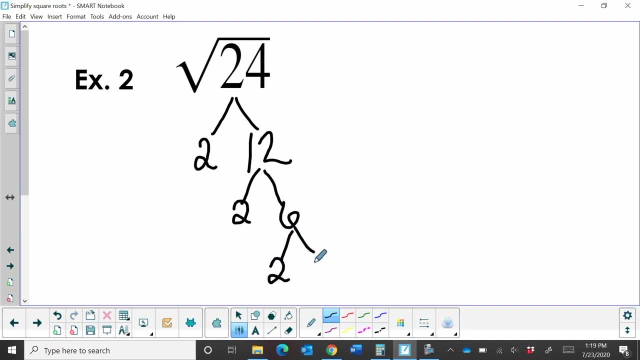 So let's, Let's make this 2 times 3.. Now my prime factors. if I write all my factors out, I have 2 times 2 times 2 times 3.. Okay, now I'm looking for, since this is a square root, 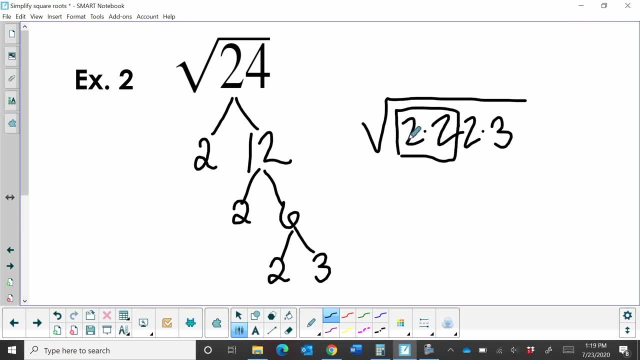 I'm looking for pairs. Well, 2 times 2 is 4,, so the square root of 4, which is this: 2 times 2, is 2.. So I'm going to pull this out, Okay. well, these are not pairs. 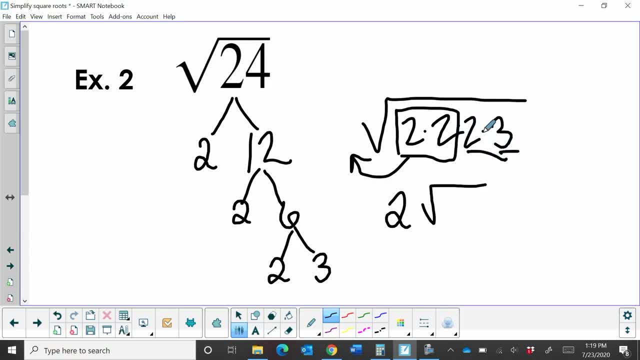 2 and a 3, they don't have a pair under the radical, So I just go ahead and multiply those back together and that's 6.. So the square root of 24 simplifies to 2, square root of 6.. 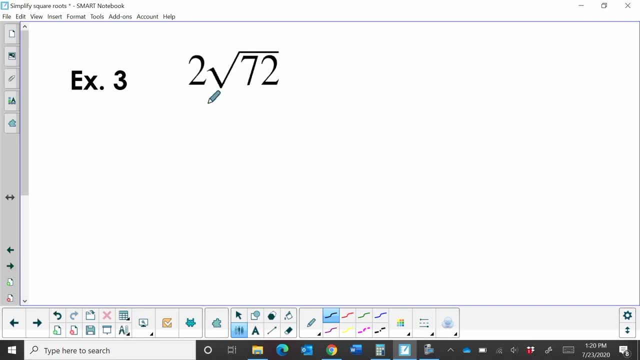 So now let's look at one more example where I have a coefficient in front of my radical. So let's start simplifying. I'm not going to ignore the 2 for a moment, and I'm just going to simplify what's under the radical. 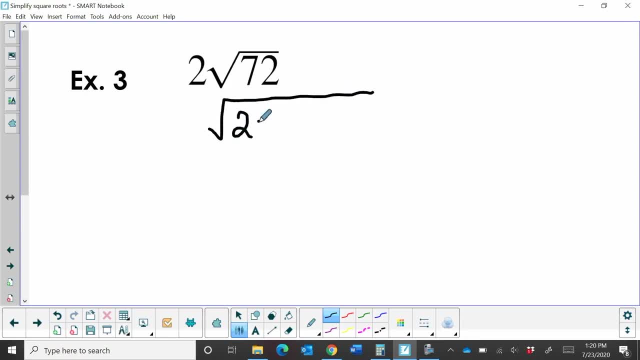 Okay, 72 factors to 2 times 36.. Again, because I have an even number, I have another even number: 2 times 18.. Well, I've already simplified 18, so I've already done this one: This one's 2 times 9, and 9 becomes my 3 times 3.. 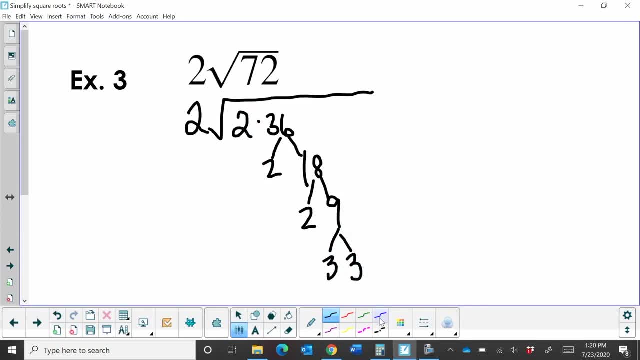 So this diagonal, This diagonal right here is- I'll circle it in blue so you can see my diagonal here- All these are the prime factors for 72.. So now I just need to pair them up. So let's pair them up. 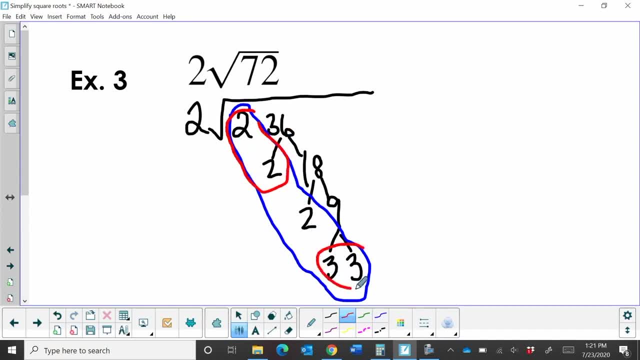 So there's a pair that's going to come out as 2, and here's a second pair that's going to come out as a 3.. So, to simplify this, I already have a 2 in the front, so I'm going to bring that over. 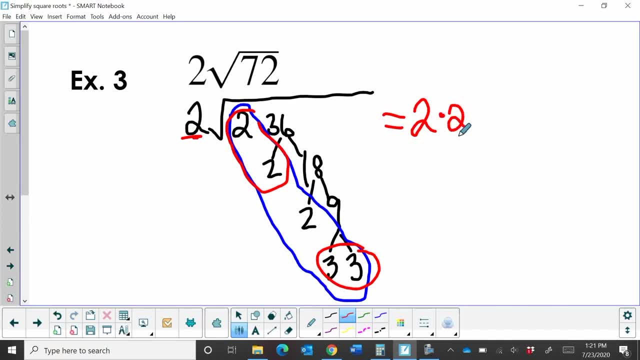 Out of this pair. I'm going to bring out a second 2, out of this pair, because that's really 9, so the square root of 9 is 3,. I'm going to bring out a 3.. Then I have to think about, well, what's not paired up?